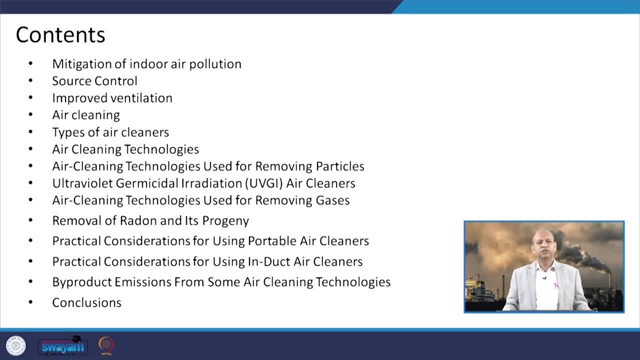 technologies, different kind of technologies like removing particles or using ultraviolet germicidal irradiation, UVGI. air cleaners, And then air cleaners, And then air cleaners, And then air cleaners. Air cleaning technologies which are used for removing gases, removal of radon and its. 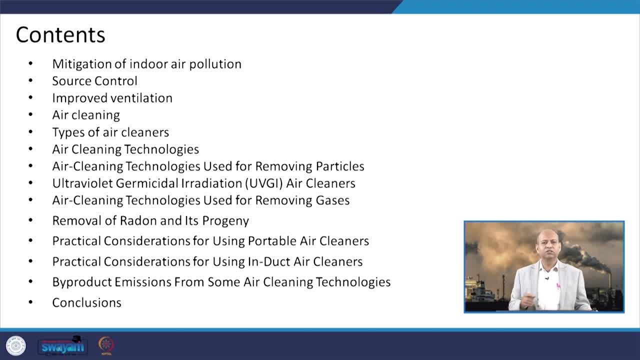 progeny and other products. practical considerations for using these portable air cleaners or induct air cleaners, because there are issues- means it is not always true that air cleaners will be very nice in handling to remove air pollution Sometimes if we are not maintaining them properly. 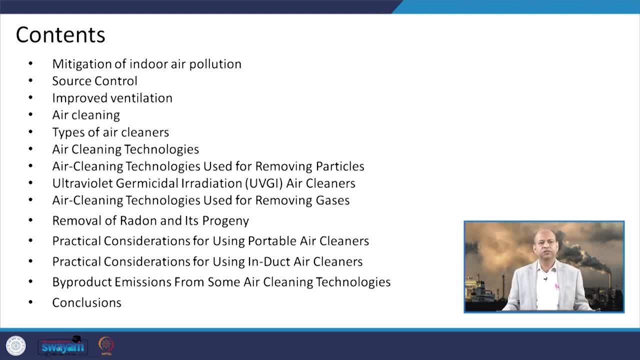 then they can be also sources of indoor air pollution. basically, Then, byproducts and products and emissions from some air cleaning technologies. as I said, that if we have to maintain them properly, otherwise there can be additional sources from these controlling devices. if we do not maintain, we do not repair them timely and then we will go for conclusions. 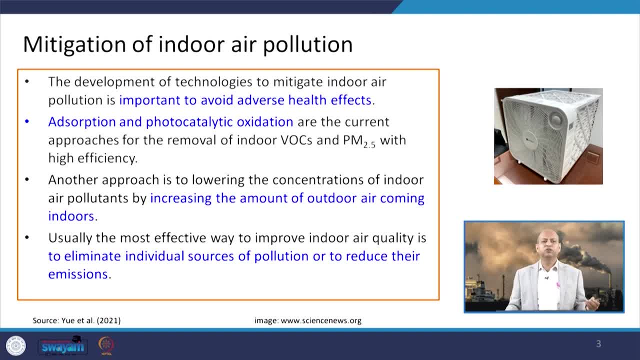 So when we talk about mitigation of indoor air pollution, why it is required. so the development of technologies which are needed for mitigating indoor air pollution is very important because you know it, otherwise the indoor air pollution can result into several kind of health effects or adverse health effects. I would say So to avoid that kind of situation, it is necessary. 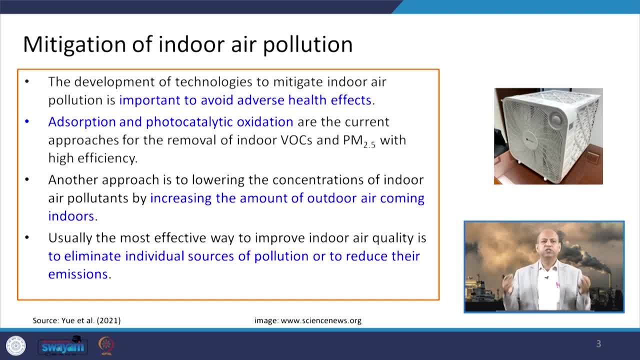 to employ certain technologies to mitigate or to control or to remove, to reduce the indoor air pollution levels. Then there are several techniques, but adsorption and photocatalytic oxidation. these are, you know, the current approaches which are, you know, kind of popularly. they are used for removing indoor VOCs, volatile organic compounds. 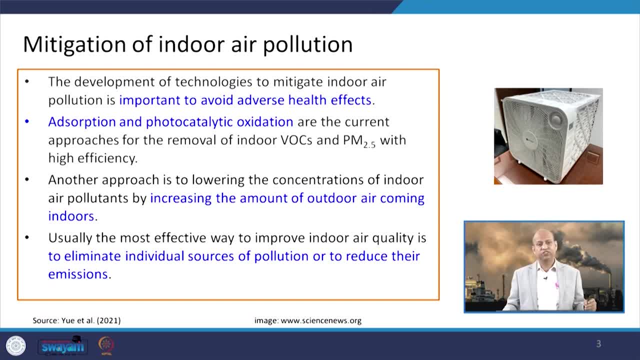 and fine particles like PM 2.5 with high efficiency. These adsorption and photocatalytic oxidation. these two processes are very popular in that sense, But there are another approach, like lowering the concentration of indoor air pollutants by increasing the amount of outdoor air coming. 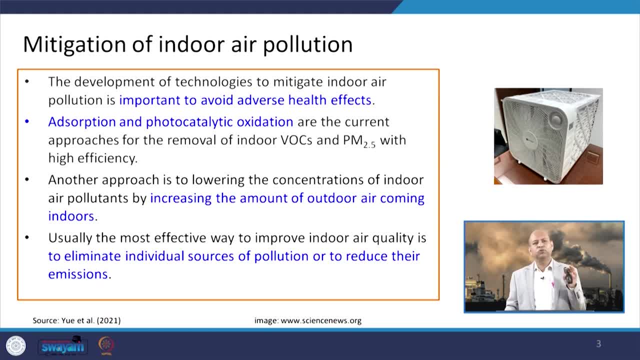 indoor through ventilations. But you know, it is a tricky thing because if outdoor air pollution, If the indoor air quality is not good, then polluted air may enter into the indoor environment. So we have to first see that the outdoor air must be clean. only then we can go for this. 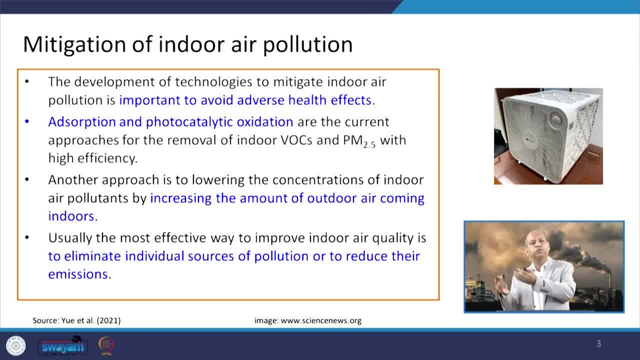 kind of situation where we increase the amount of inflow of the outdoor air to indoor environment, Then it can improve the indoor air quality. otherwise, if the outdoor air quality is not good, then this is not the right approach. Usually the most effective and, you know, successful way to improve indoor air quality is to eliminate 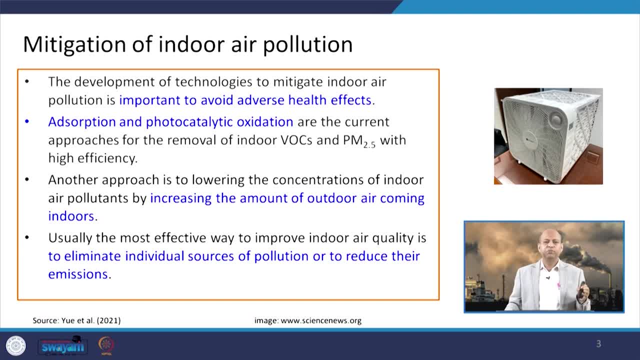 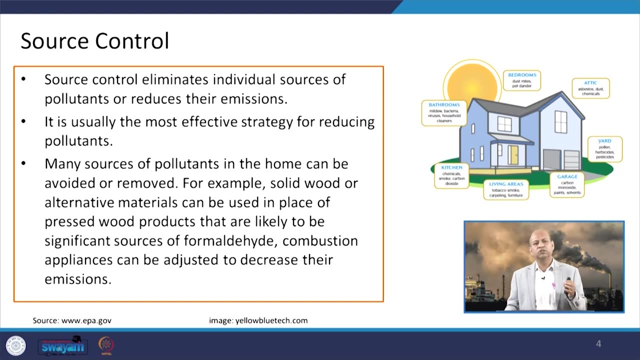 individual sources of pollution or to reduce their emissions inside the indoor environment itself. There should not be any source means. at the source itself we should do something which can eliminate these emissions of air pollutants. So basically, the source control mechanism eliminates individual sources of pollutants or it reduces it, their emissions. 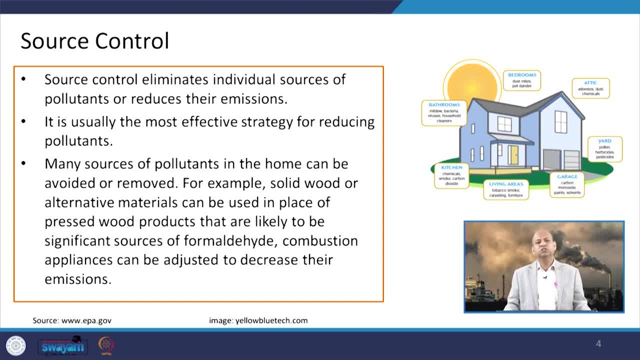 and this is usually the most effective strategy for reducing pollutants inside the microenvironment. Many sources of pollutants in the home can be avoided or removed, for example, like if we these solid wood or alternative materials can be used in place of the pressed wood or those you know, plywoods or boards, etc. which are basically significant sources of formaldehyde. 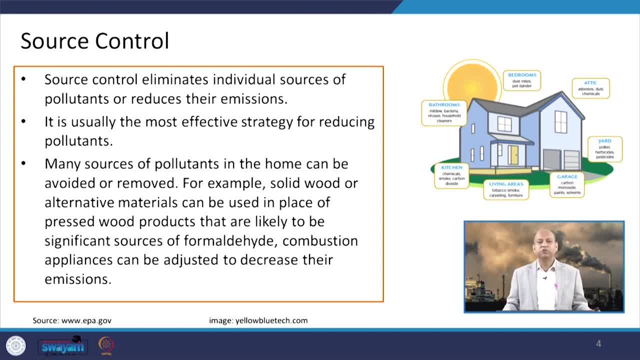 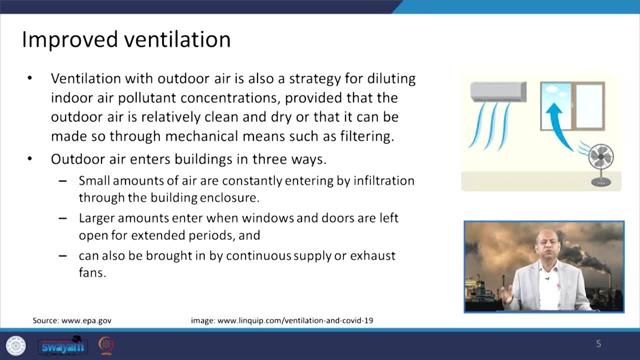 and the combustion appliances can be adjusted to decrease the emissions in kitchen, etc. So those kind of things we can accomplish through interventions of technology, Thank you, Thank you. In the next session we will talk about the use of different products. So first we will talk about the use of different products and then we will talk about the use. 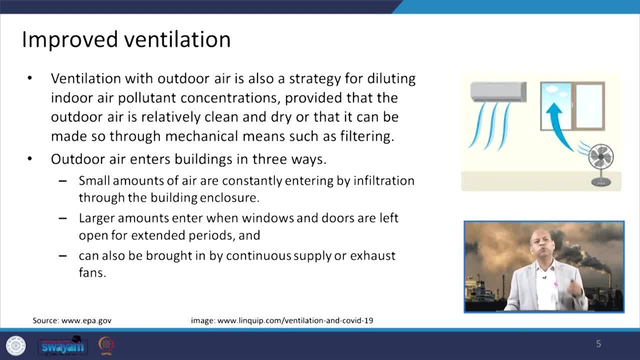 of different environmental interventions. So the first one is the use of different environmental interventions, or some changes in the usage of different products. Well, when we talk about improved ventilation, so the ventilation with outdoor air is also a strategy for diluting indoor air pollutant concentration. but, as I said, in that case the 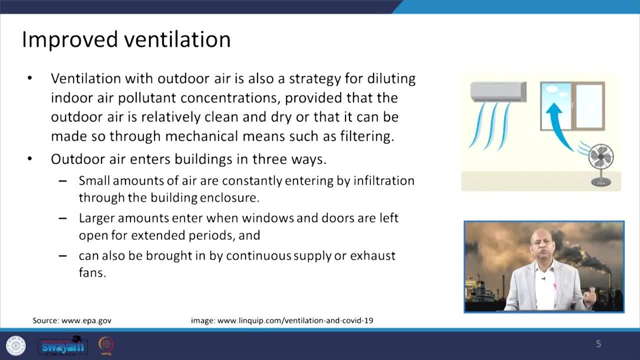 outdoor air must be clean with respect to the indoor environment, provided you know it is relatively clean and dry means it should not be humid. also because humid air, if it enters into the micro environment, indoor environment, then there are certain changes that are going to be there. 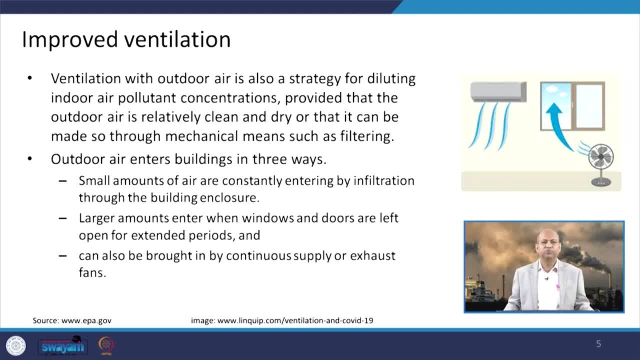 several issues, like moulds or many kind of microbes can grow in the humid environment. So the outdoor air is clean and dry. only then it is a good strategy to bring it inside the micro environment of indoor environment. Well then, outdoor air enters buildings in three ways, basically like a small amount of 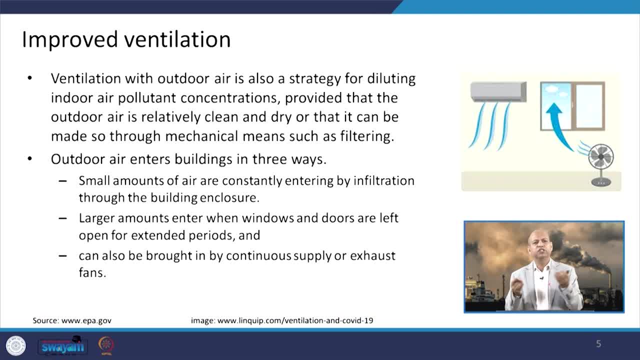 air constantly enters through various infiltration, building enclosures etc. Then large amount can enter through windows or doors whenever we open them and then it can also be brought by like continuous supply or exhaust fans means that kind of mechanism can be developed where certain fan are there only for bringing air inside the indoor environment. 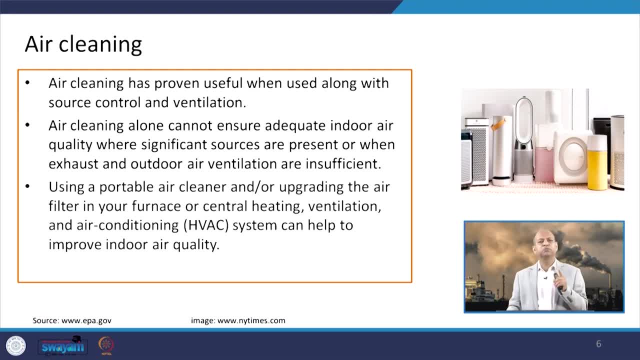 only, But as I repeat again that the outdoor air must be clean and dry, only then it is better to improve the air quality of indoors environment. Well then there are. There are air cleaning mechanism, like air cleaners or these various devices are there, portable as well, as you can have mounted in the ducts, etc. 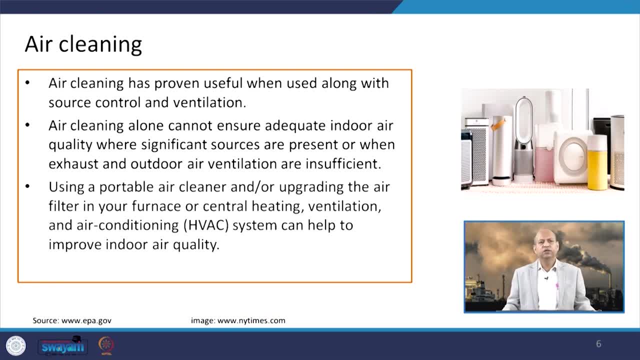 So this air cleaning has proven useful. basically, and it is used along with the source control and ventilation, Air cleaning alone cannot ensure adequate indoor air quality where significant sources are present, Because then sources may be very dominating, So the air pollution emissions. so when exhaust and outdoor air ventilations are insufficient, 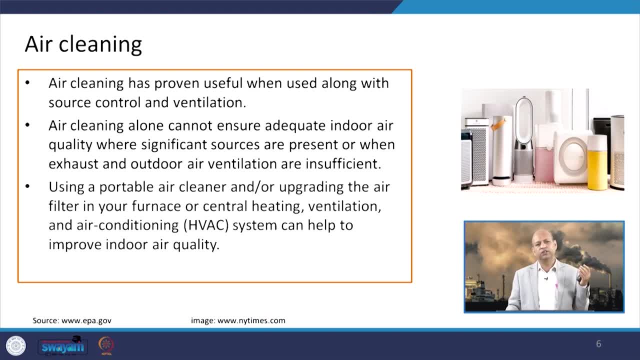 then alone this air cleaning may not be so effective. So it is a kind of integrated approach. You also have those ventilation mechanism. plus, you also do air cleaning, So using a portable air cleaner or upgrading the air filters which are used in the furnaces. 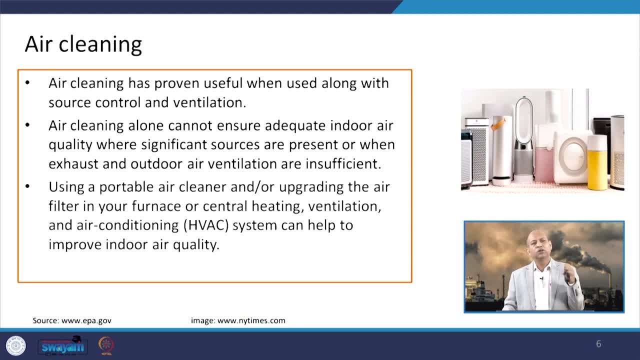 because indoor environment does not mean only the domestic or residential environment, So it is a kind of integrated approach. So it is a kind of integrated approach, So using a portable air cleaner or upgrading the air filters which are used in the furnaces. 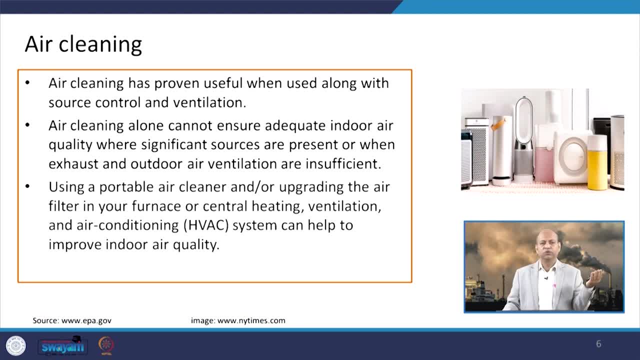 For example, travel room scale houses. indoor environments are there in factory spaces, In industries. there are these occupational spaces where workers are working, So those indoor environments are also needed to be cleaned. So the heating, ventilation and air conditioning as VSE. this system is there always for cleaning. 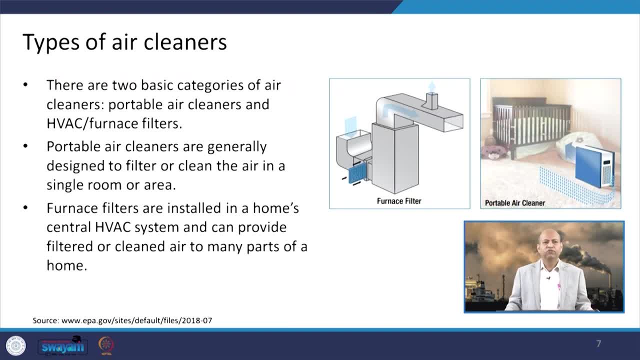 the air and to improve the indoor air quality. Well, so there are two basic categories of air cleaners, like portable air cleaners and these HVAC, these heating ventilation and air conditioning at the furnaces and other kind of locations. So portable air cleaners generally used where you can have these kind of filter mechanism. 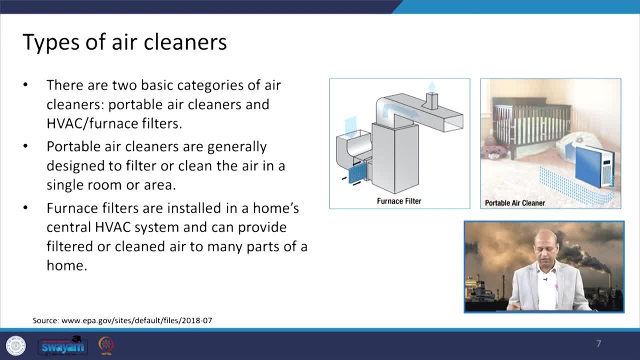 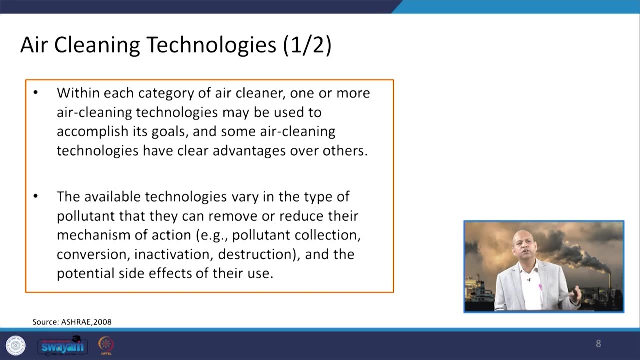 where it sucks air and then passes through after capturing particulate matter etc. Furnace filters are there in these occupational spaces, in the factories etc. So those kind of HVAC systems can also be used. But within each category of these air cleaners, one or more air cleaning technologies may. 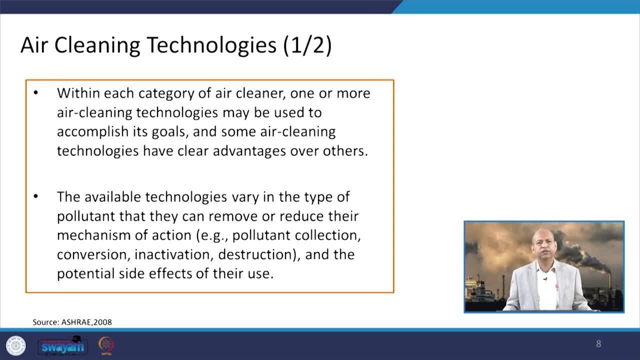 be used to accomplish the aims of better air quality, and the available technologies can vary in the type of pollutant. when some gases has to be controlled, then or reduced, then other kind of technology can be used. when particulate matter is the target, then some other way of removal of these mechanism can be employed. 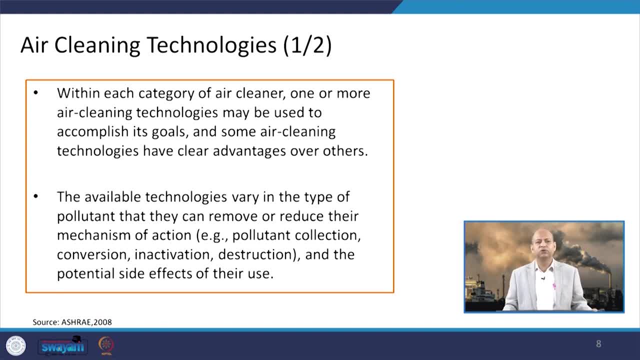 So, like You know, pollutant collection or conversion or inactivation, destruction, all these kind of mechanism can be there in different technologies and there may be some potential side effects. also we have to see like filters if we do not change of the these portable air cleaners. 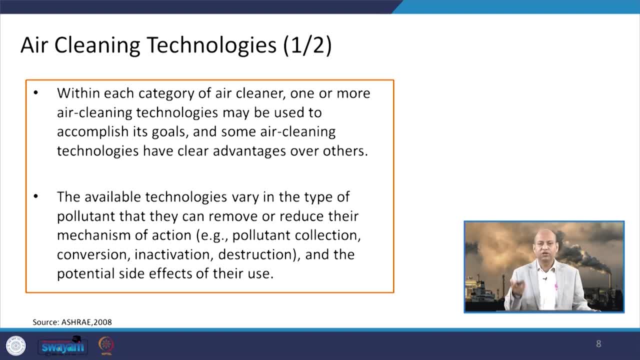 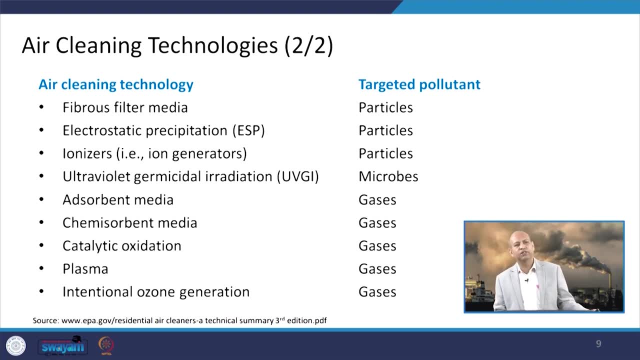 those filters can be sources of the indoor air pollution. So rather than cleaning the air, they can pollute it. So that has to be kept in mind. well, when we talk about different technologies of air cleaning, then You can see- this is the list- like fibrous filter media can be used, or electrostatic. 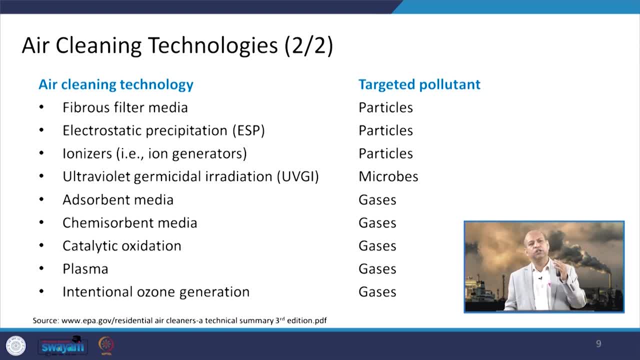 precipitation ESP can be used, which you have studied. we have studied in the like industrial air pollution control mechanism, So the small size ESPs can be used in indoor environment also. then ionizers can also be there. I am repeating it again that please do not feel that only the residential rooms 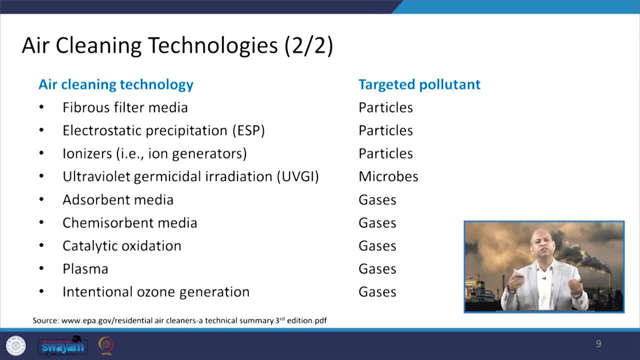 or those houses are the indoor environment. Indoor environment can be of various kinds, Like Big factories or libraries or museums or whatever built environment is there where people are working. So those large size indoor environments can be there and you may need you know these ESPs. 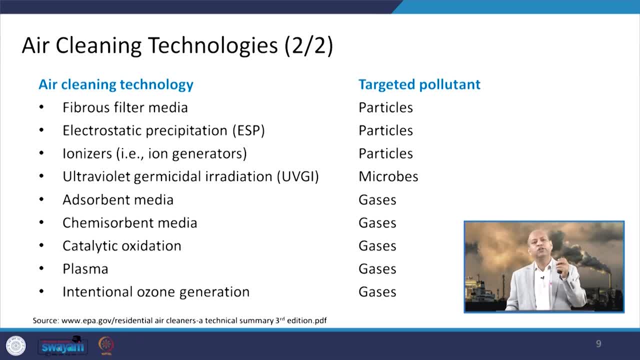 etcetera, those kind of instruments. well then, ultraviolet germicidal irradiation, UVGI, can also be used. adsorbent media can be used, or chemisorbent media can be used, catalytic oxidation: like You know, These are the way catalytic things are used in exhaust pipes of vehicles. so similarly, 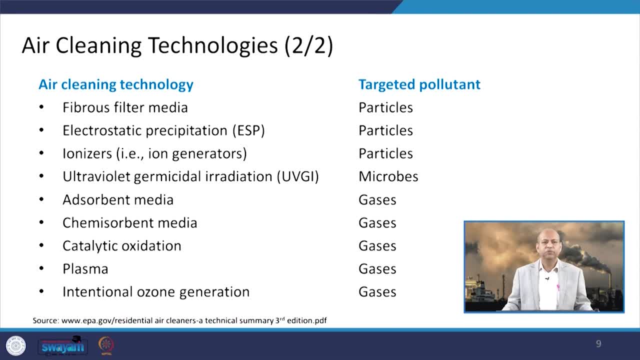 in indoor environments also. some catalytic oxidation mechanism can also be used. then plasma related technology is there. Then there is like ozone generation, because ozone is an oxidizing agent. So for oxidizing those gases which are pollutants, ozone can be generated and that can be used. 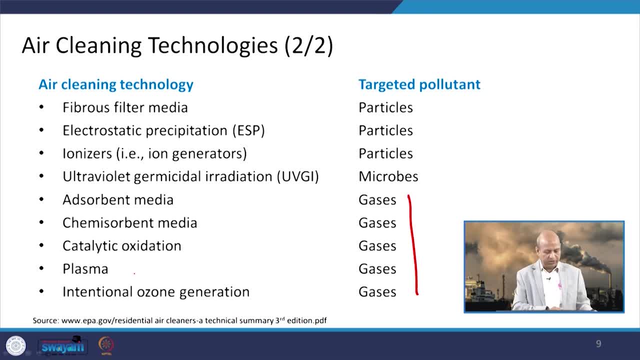 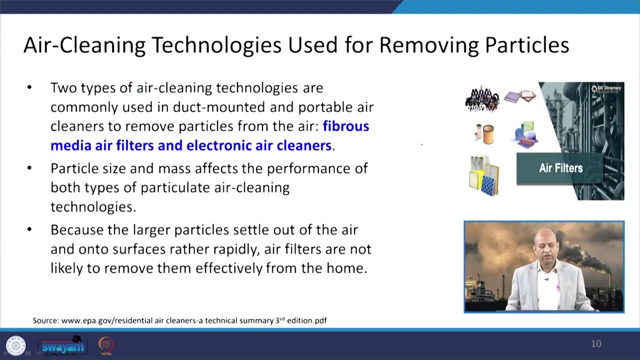 So for gases, you know these adsorbent media, chemisorbent catalytic oxidation, plasma and intestinal ozone, these are the better technologies. for microbes, these UVGI, and for particles, filter media or these ESPs and ionizers can be used most effectively. Well, the two types of air cleaning technologies are commonly used in duct mounted ducts are: 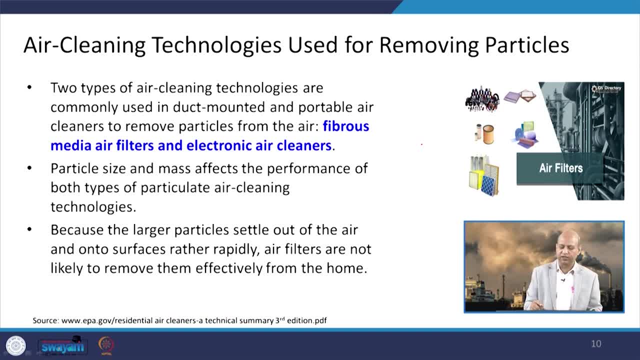 there and then portable air cleaners to remove particles, like fibrous media, air filters and electronic air cleaners. So these are the two types which are very popular And power cleaners. And particle size or the mass, you know, of the particles, they, you know, influence the 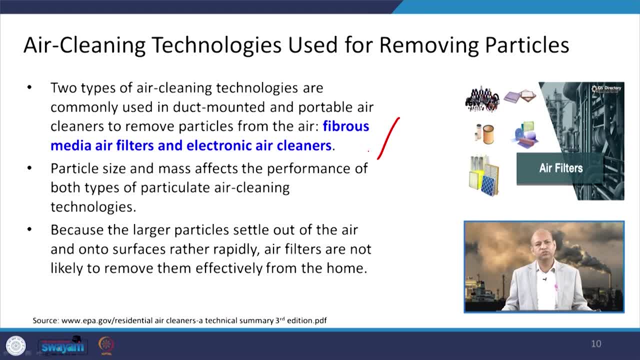 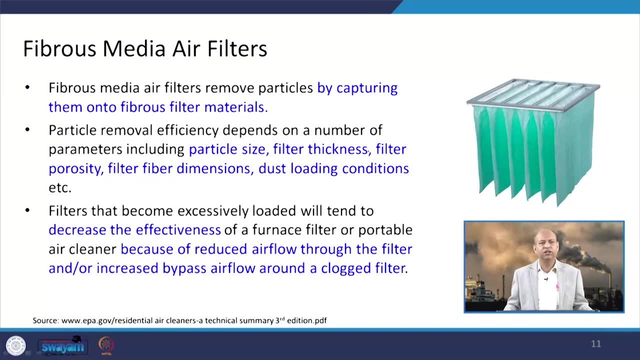 performance of these kind of air cleaning technology? basically Because the larger particles settle out of the air and onto the surfaces rather rapidly, so the air filters are not likely to remove them effectively from the home. So that is why you know other kind of technologies are employed. 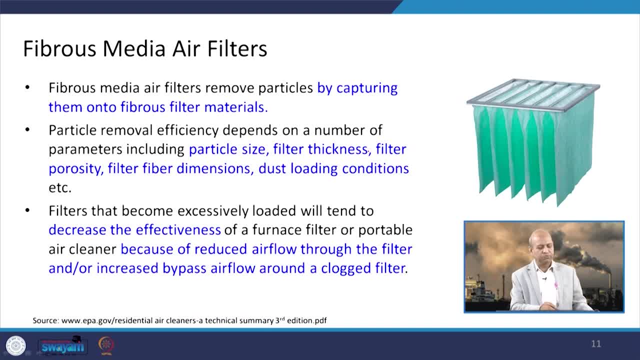 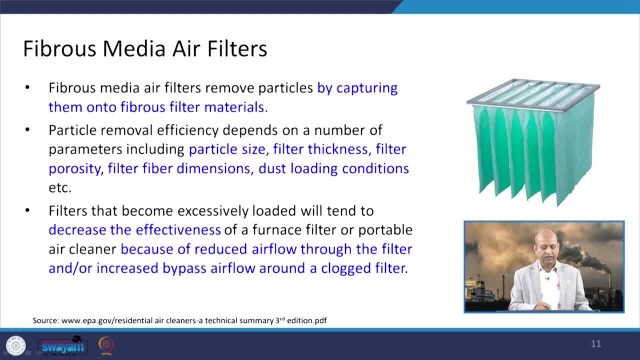 So those kind of fibrous filter materials are there and you know, depending upon the particle size or fibre thickness, then filter porosity and filter fiber dimensions, dust, loading conditions, all these things influence the efficiency of the removal of these particles And you know these filters that become excessively loaded will tend to decrease the efficiency. 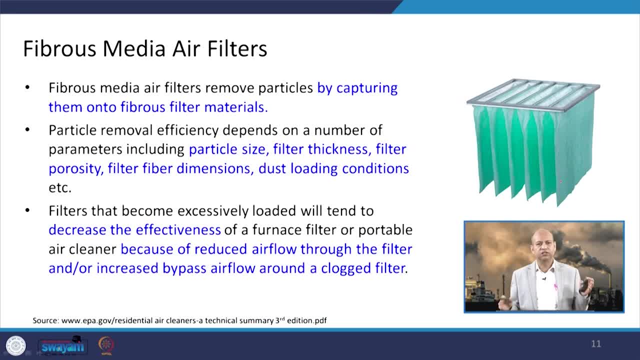 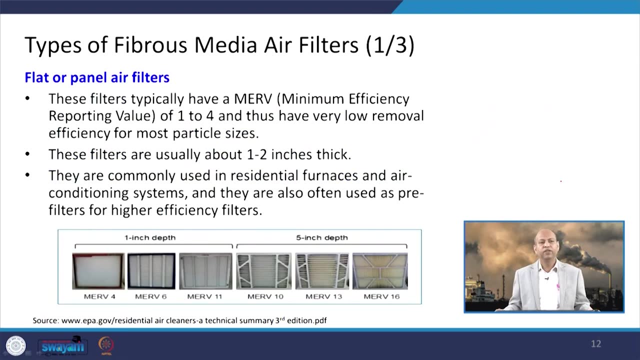 is the efficiency or effectiveness of the filters. basically, when porosity is less And because of, you know, reduced air flow through the filters and increased bypass air flow around, a clogged filter can rather pollute the indoor environment instead of cleaning it. So these kind of things we have to keep in mind to do better maintenance or frequently. 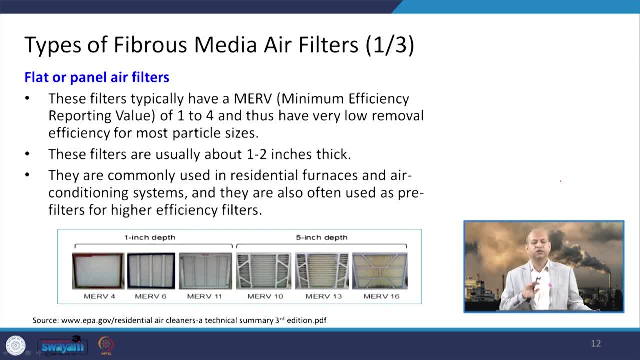 we should do something to remove those clogging kind of situations. Well then, flat or panel air filters can also be there. So this is again. typically they have this MERV minimum efficiency reporting value 1 to 4.. So different values are there depending upon their efficiency. then thickness can also. 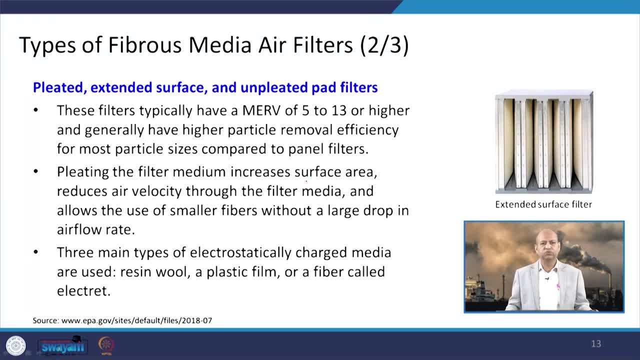 be a matter of concern. So all those things we have to see plus at the same time, you know, the splitting of these pleats, of these filter media, can also give us better surface area and it can reduce a lot is the air velocity and better efficiency can be achieved. 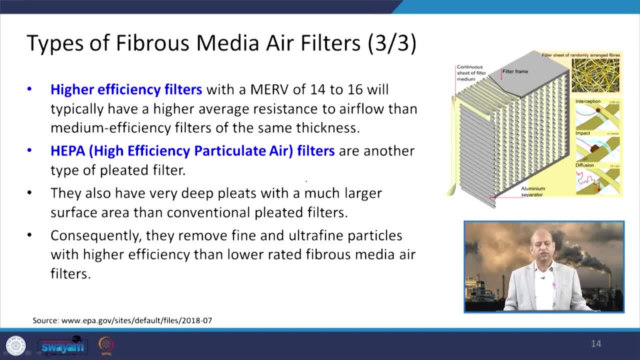 Well, when we talk about, you know, efficiency of these fibrous media, higher efficiency with the MERV of 14 to 16 will typically have a higher average resistant to air flow than medium efficiency filters. So that again, so it need more power. you can say. 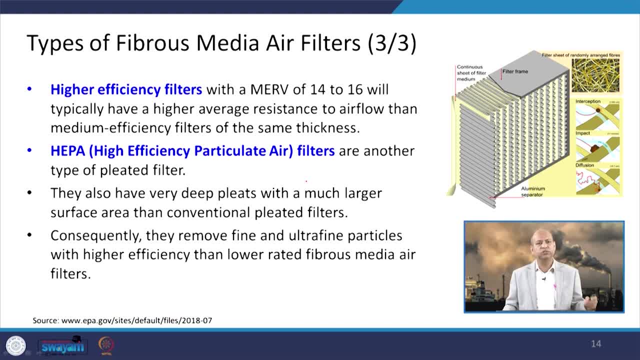 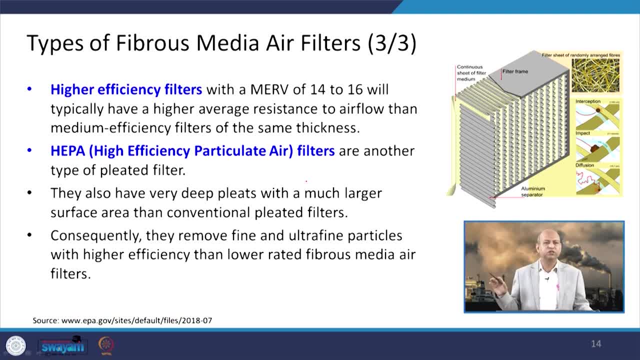 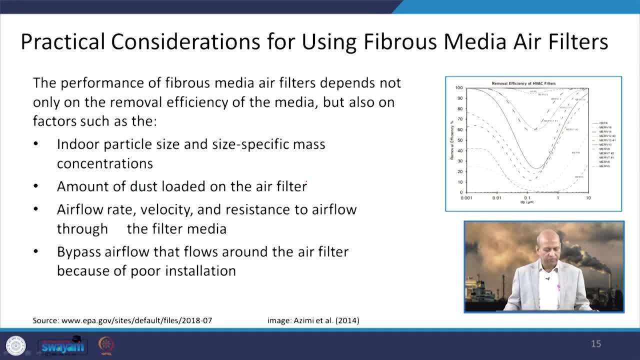 particles very efficiently in that way. Well, when we talk about, you know, these practical considerations for using fibrous media air filters, because if you do not use them properly, then rather than increasing the air quality, making air quality better, So you know, you know, deteriorate it. 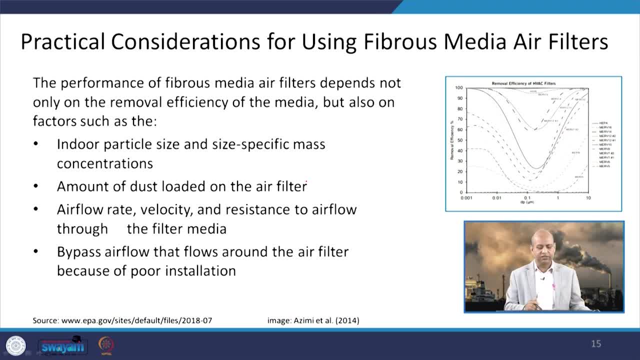 So then, to indoor particle size or size, specific mass concentrations, amount of the dust loaded on the filter, and then air flow rate, velocity and bypass air flow that flows, you know, around the air filters. all these things have to be kept mind and the optimization has to be done. 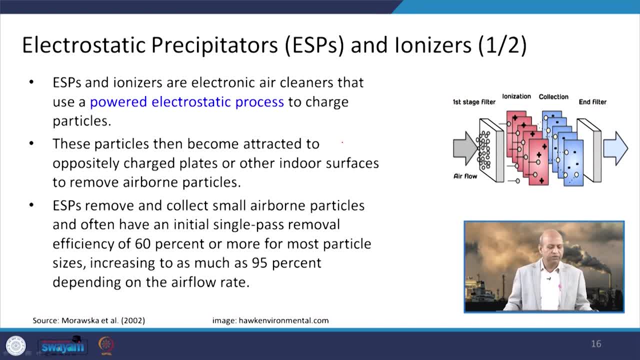 to have greater efficiency of those filters. Well, when we talk about electrostatic precipitators or ionizers, so as you know, ESPs can be used for removing particles with high efficiency, But you know they can collect small airborne particles and you know they can have efficiency. 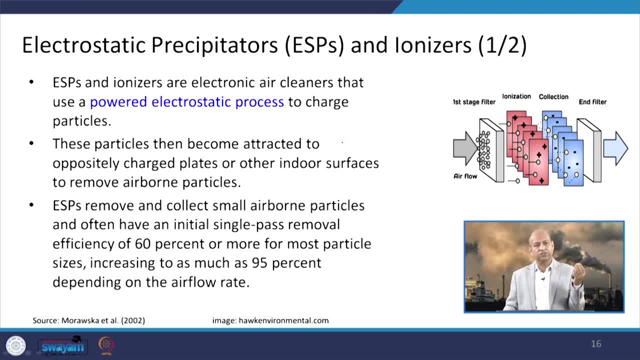 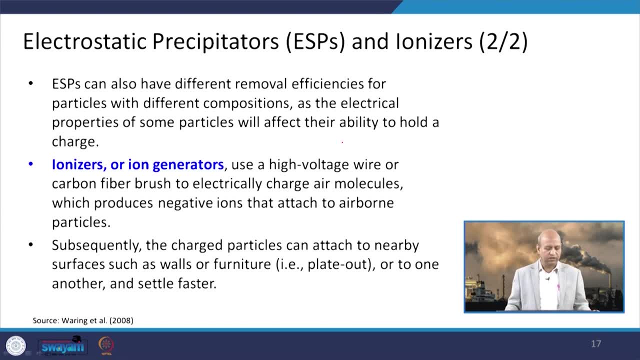 varying from 60 percent to even 95 percent, depending upon what is the size of the particles and how much path is there, how many number of plates are there? all those issues are there. Then ionizers can be there, ion generators, So they also create some situation where different of charged particles can be captured. 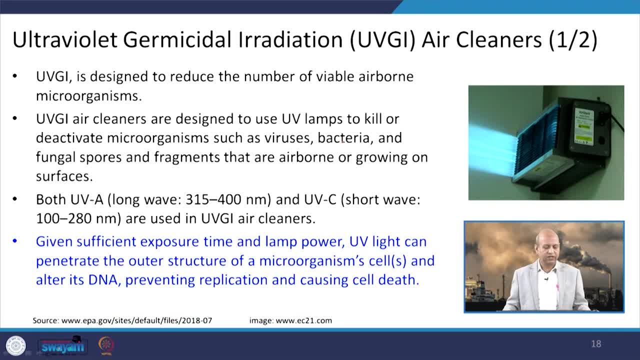 by other filters, So those plates of different charges. Well, when we talk about ultraviolet germicidal radiation, UVGI, air cleaners, you might have seen, during, you know, covid period, these UV based cleaning devices has come into the market. So similar devices are there already for you know, deactivating microorganisms such 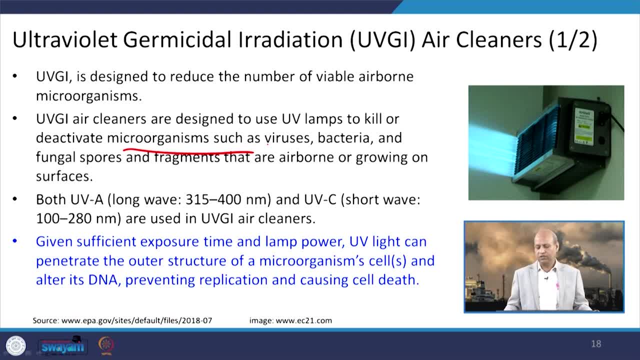 as viruses or bacteria. So those are the devices which can be used for killing these kind of microbes. Okay, So, for insufficient exposure in terms of time and the lamp power, these UV light can penetrate the outer structure of the microorganism cells and they can alter its DNA. 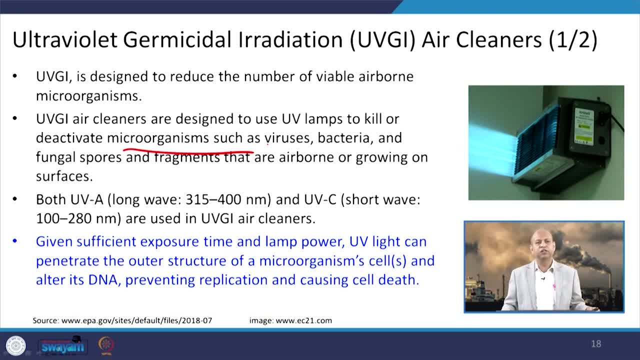 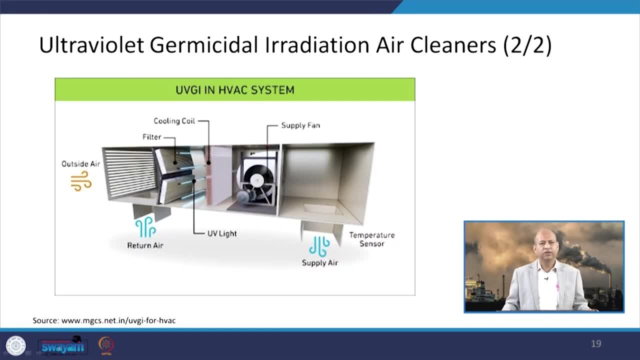 So they can prevent its replication or further multiplication, and then they can cause the cell death, So that way the bacteria or virus can be killed. Well, the ultraviolet, these UVGI kind of air cleaners. this is the diagram which shows how it is installed in the indoor environment. 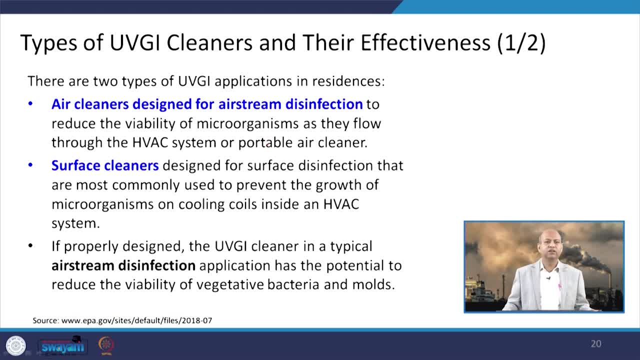 They can be different types of these UVGI cleaners, like air cleaners designed for airstream disinfection, where you know the those rays- UV rays- are passed through the air and whatever microbes are floating into the air, they will be killed. Then surface cleaners, like when we put something and then in the box there is this UVGI's. 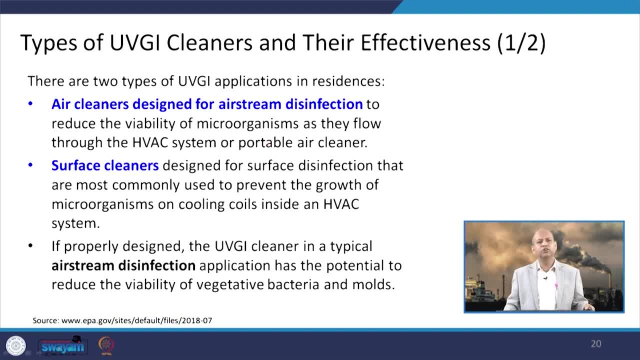 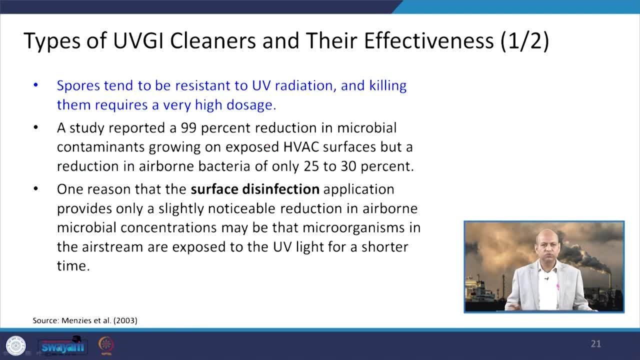 those rays are there, radiation are there, then they kill. So those kind of, you know, devices which are cleaners for the surface, Okay, They are more efficient, basically, in comparison to the airstream. So you know more time is needed for airstream cleaning. 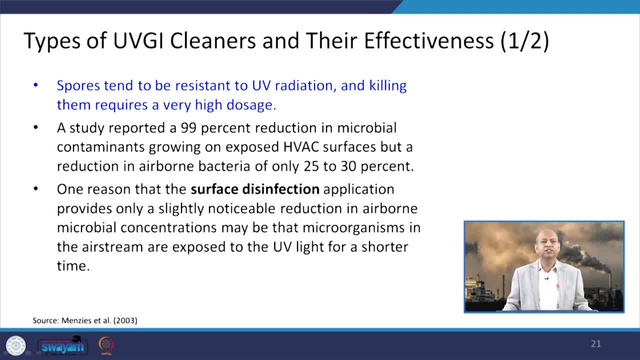 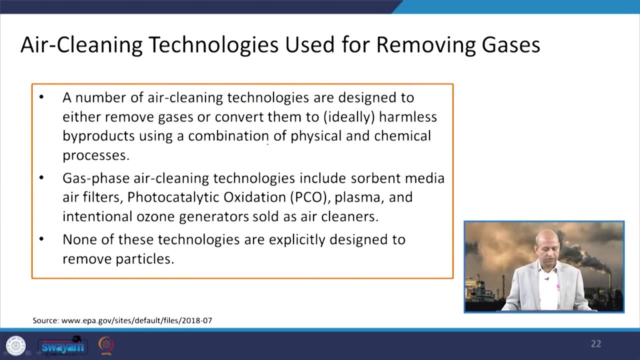 You know, these spores tend to resistant to UV radiation and killing them requires a very high dosage. So, depending upon what kind of indoor environment is there, we have to settle down with the intensity of the UV rays as well as the time of the exposure for those cleaning purposes. 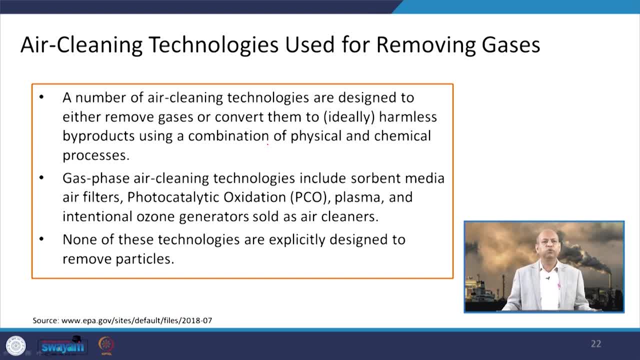 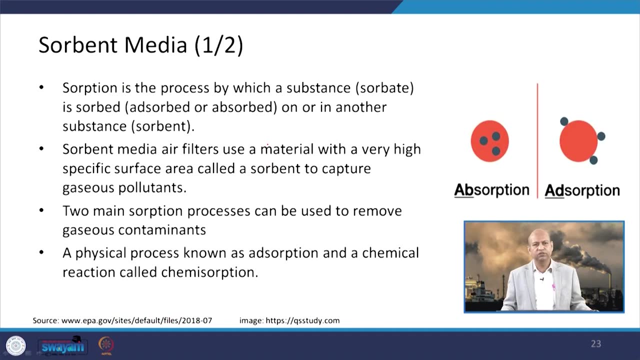 Well, when we talk about like technologies for removing gases, Then number of technologies are there, like gas, phase air cleaning technologies can be there for like photocatalytic oxidation, PCO can be there, plasma based technology can be there or ozone generation. So we will see one by one. like absorbent media means absorption can be there, absorption. 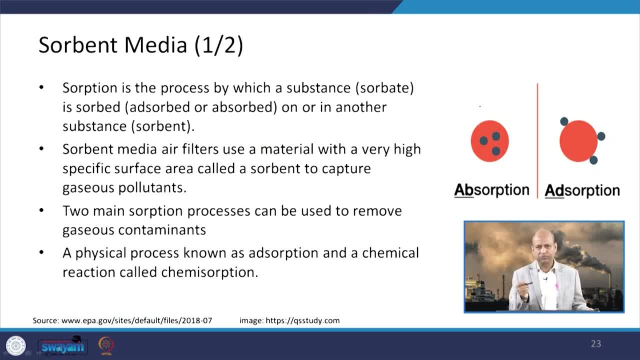 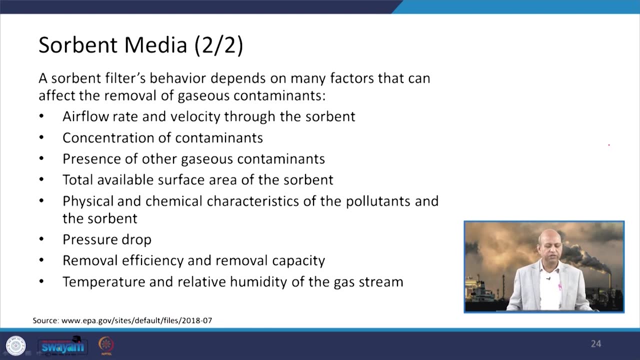 or adsorption. So absorption means inside, it can absorb. some chemical reactions can be there. adsorption maybe through attraction, physical attraction, it can keep on the surfaces. So though both the phenomena are used for- Okay, For removing those gaseous pollutants. well, you can see these absorbent media or filters. 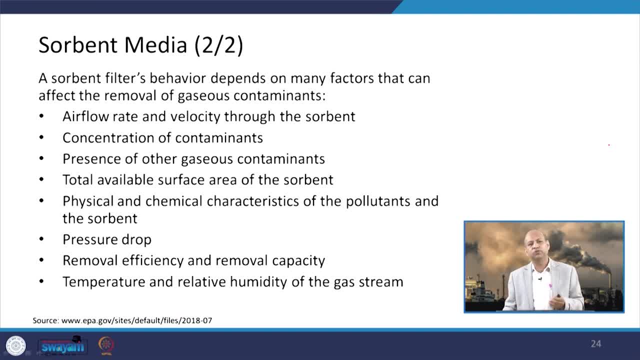 behavior depends on many factors like air flow rate or velocity through the this absorbent media. Then what is the concentration of the contaminants or pollutants? presence of other gaseous contaminants rather than in addition to the gases which we want to remove? Then total available surface area for adsorption purpose. physical chemical characteristics of 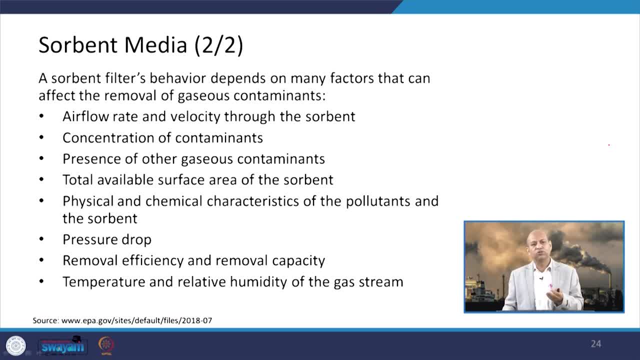 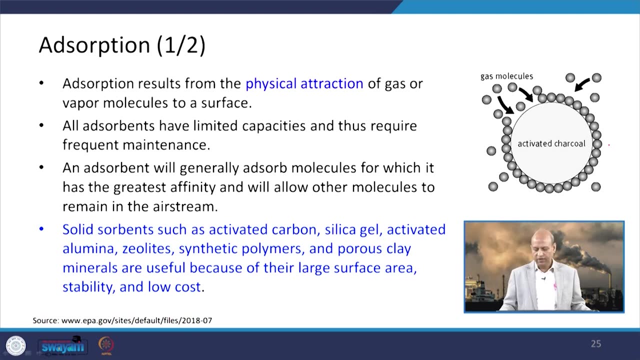 the pollutants And the absorbent media. then pressure drop or removal efficiency, removal capacity, temperature and relative humidity of the gas stream. all these issues are there, or factors are there which influence the efficiency or performance of these absorption or adsorption related cleaning mechanism. So in adsorption you can see the physical attraction of the gases which can captured. 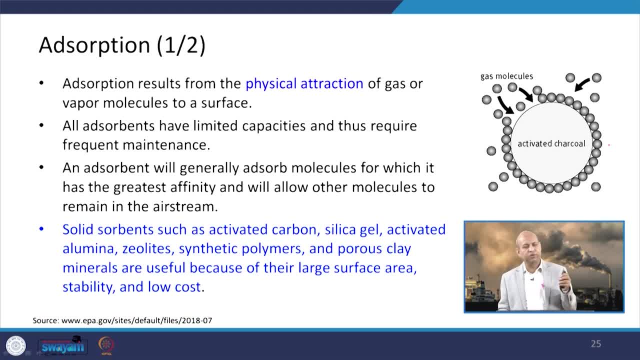 on the molecules of the surfaces: Okay. And the solid absorbent, such as activated carbon, silica, gel, activated alumina, geosynthetic- Okay. So these are the factors which influence the efficiency or performance of these absorption or adsorption related cleaning mechanism. 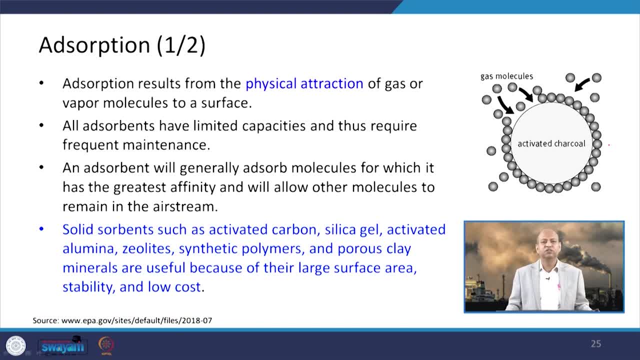 So the absorption there, because for example you can say begging have obviously the absorption of the particles, activity which can captured on the acids inking process which are the molecule sub dormant application. also there, the squeezing those rise up the consumables. Yes, on the Reinforced. 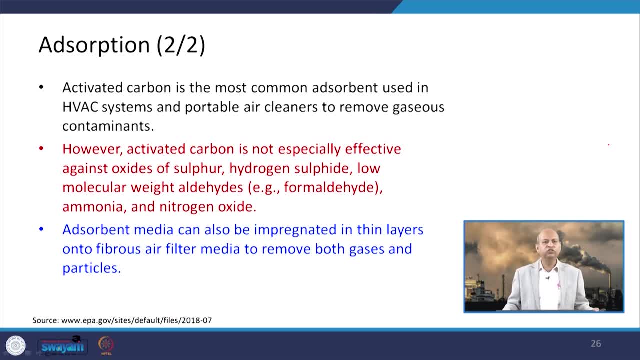 Solid, you can also apply it and also without particulate по useful. It can also be like easiest way to remove gas and particulate is actually a process before it, so they not just appear Okay. But we have to be very cautious because the activated carbon is not especially effective. 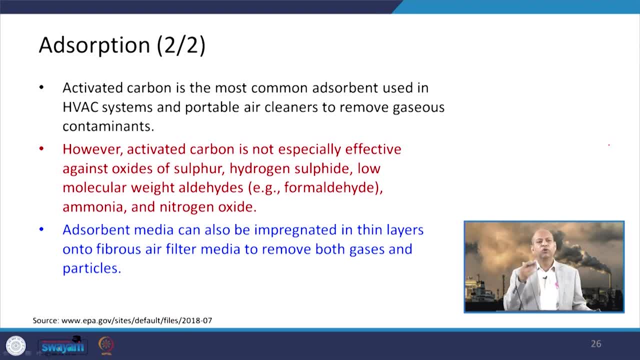 against oxides of sulphur or hydrogen sulphide or low molecular weight aldehydes and even ammonia or nitrogen oxide. So depending upon the nature of the gaseous pollutant we have to use, which kind of adsorption material we can use. 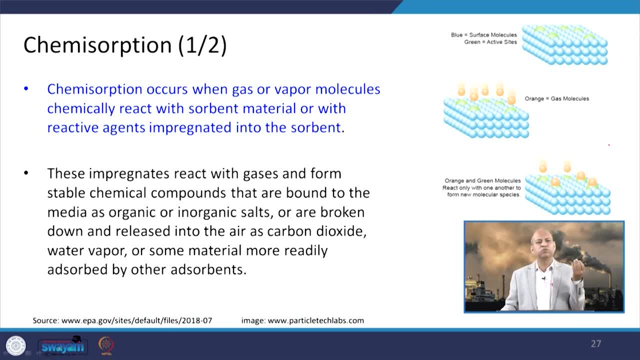 Then chemisorption can be there, where it can have gas or vapour molecules. chemically it can react with the sorbent material or with the reactive agents, this impregnated into the sorbent. So the chemical bond is there basically. that is why we call it chemisorption. 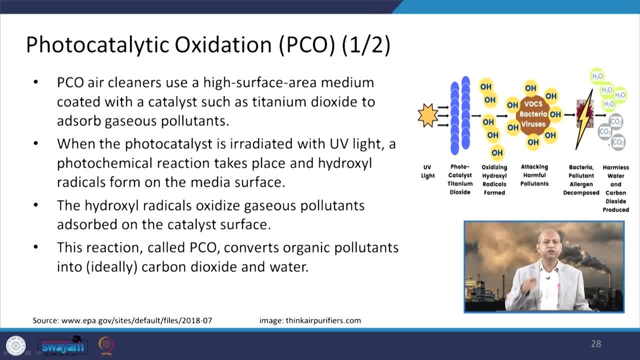 Then there can be like photocatalytic oxidation, as I gave that example, in vehicular exhaust. 3-way catalytic converters are used, So that way also in PCOs, this photocatalytic oxidation in indoor environment. they can use a high surface area medium coated with a catalytic such as titanium diuretic. 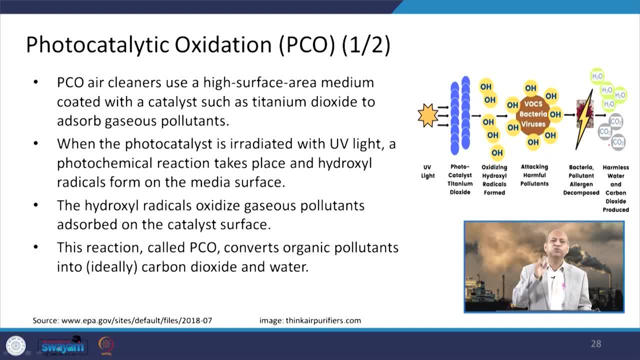 So when the photocatalyst is irradiated with ultraviolet light, a photochemical reaction takes place and these hydroxyl HO, hydroxyl radicals, they are formed on the media surfaces and, as you know, these OH radicals, or hydroxyl radicals, are very quickly they oxidize whatever. 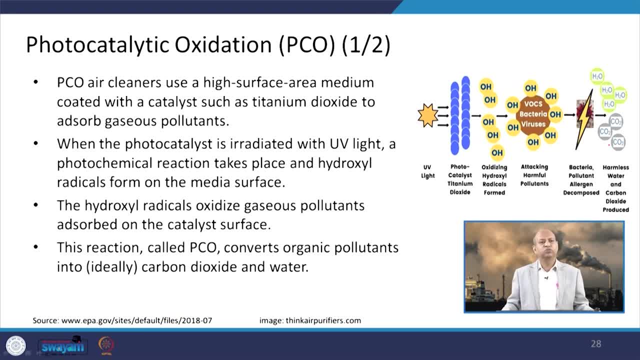 they come into contact, So these hydroxyl radicals, they can oxidize gaseous pollutants and they can be adsorbed on the catalytic surfaces. So that way very quick reaction occurs, and this reaction, which is called PCO, this converts. 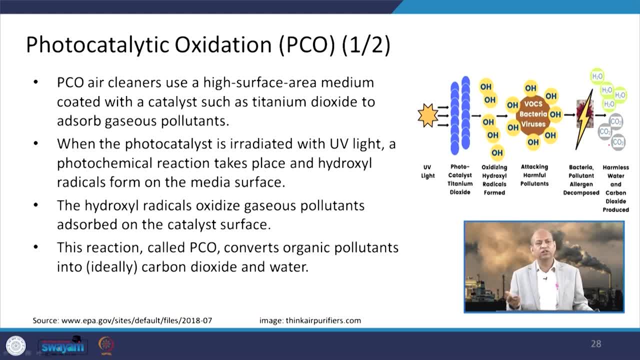 the organic pollutants into carbon dioxide or water, So with they are harmless. in the sense they are not pollutants. but of course both are greenhouse gases. So from that perspective, although things are there, issues are there, but from health point of view at least they are not problematic. 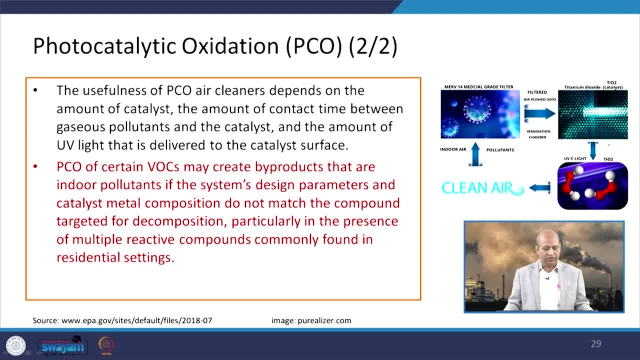 Well, when we talk about further in this PCO technique. So the usefulness of these PCO air cleaners depends upon, you know, this amount of the catalyst and the amount of contact time between gaseous pollutants and the catalyst And the amount of UV light that is delivered to the this catalyst surface. 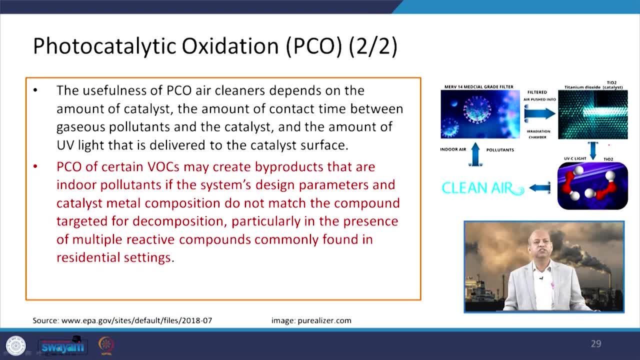 So all these factors are there for influencing the efficiency or efficacy of the PCO devices And the PCO of certain VOCs, like volatile organic compounds or hydrocarbons, may create some byproducts which are, you know, indoor air pollutants In it also. 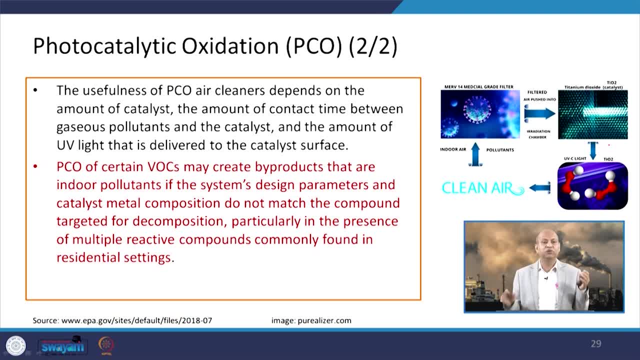 Ok itself. So if the system design parameters are not good, rather than removing you know the pollutants, it can generate some other pollutants byproducts. So we have to be very careful in that you know handling the PCO related techniques and so it should clean, rather than you know adding some pollutants. 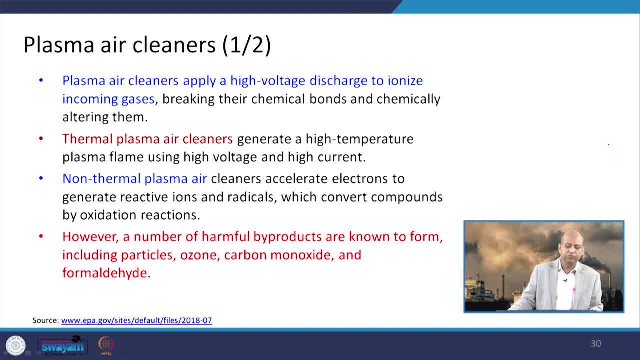 So these side effects we should be careful about. Plasma air cleaners can be there. So these, you know, in thermal plasma air cleaners can be there or non thermal plasma air cleaners can be there. So depending upon their- you know- voltage and then the radicals, we can use any of them. 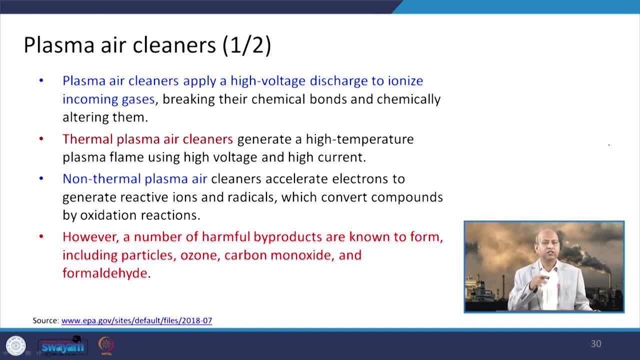 But a number of harmful byproducts. again, like in PCO, in this plasma technology also there may be, you know, some particles, or ozone, carbon monoxide, formaldehyde. they can be byproducts if we do not handle properly this technology. So these technologies are good if we are handling them properly, otherwise they may. 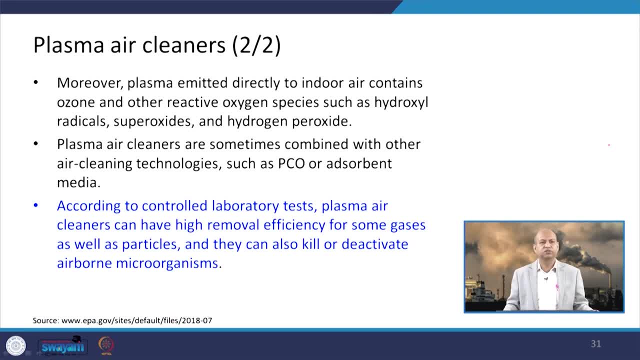 be problematic because they can also add some pollutants Well, according to the control laboratory tests. so when we use properly, this plasma air cleaners can have very high removal efficiency to some gases as well as particles, as they can also kill and deactivate airborne microorganism. 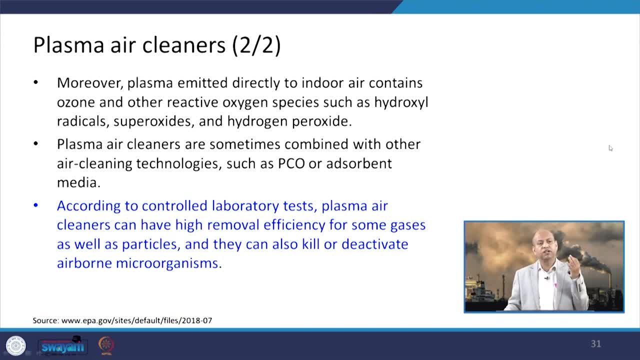 So that way, plasma air cleaners are very good, As I said, if it is, you know, used in a controlled manner, in a with a those skilled people they can use. otherwise it can be dangerous also. So you know, if we use it in a controlled way. 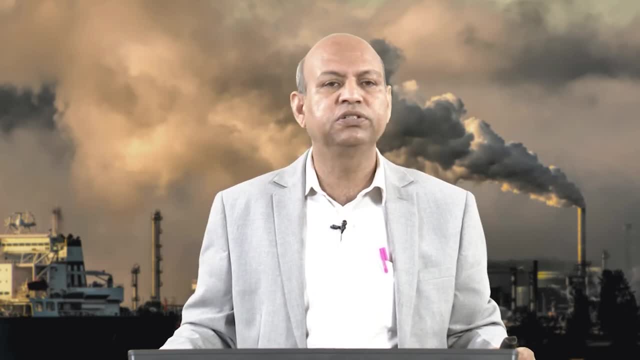 This can be done. This can be a very good technology because it can remove particles as well as gases, pollutants, and it can also kill or deactivate airborne microorganism. So skilled people or you know, personnel, are you needed for plasma air cleaners for using? 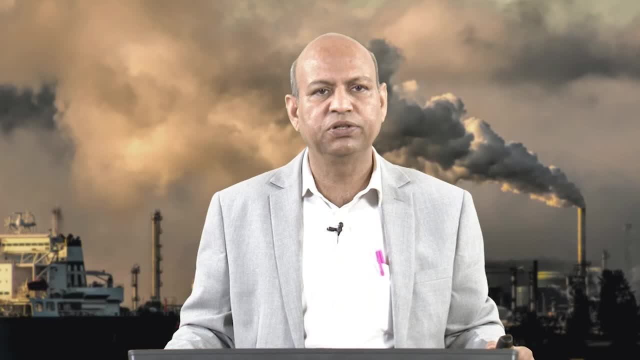 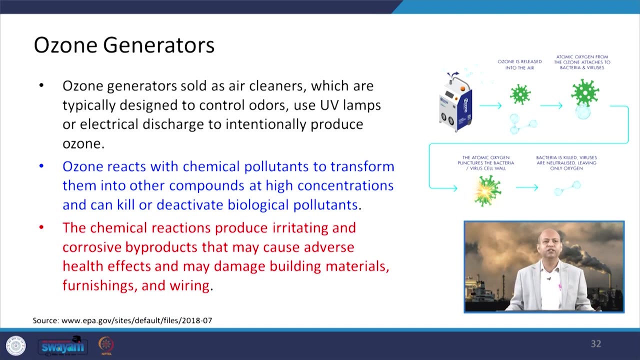 the plasma air cleaners, otherwise it can be a problematic also. we should be careful. Then there can be ozone generators and you know this also needs very careful handling. otherwise ozone itself is a problematic problem. It is a very toxic pollutant but it can be used as a oxidizing agent also, as you know. 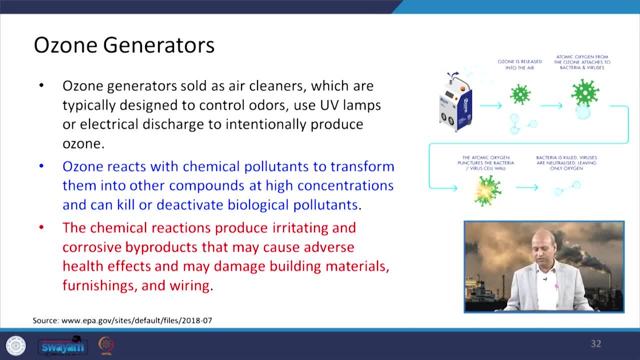 this ozone has nascent oxygen, So it can oxidize and it can clean. it can oxidize the pollutants and it can react with chemical pollutants to transform them into other kind of compounds at high concentrations, and it can also kill and deactivate biological pollutants. 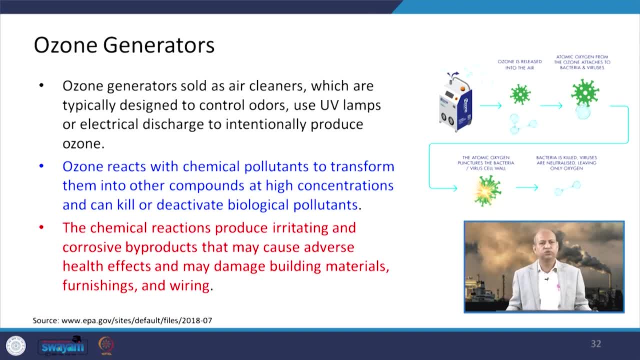 So that way, similar to plasma technology, it is also good technology. But the chemical reactions produce irritating and, you know, corrosive byproducts that may cause adverse effects. It may cause health effects and may damage building materials also or furnishing or wiring, etcetera. 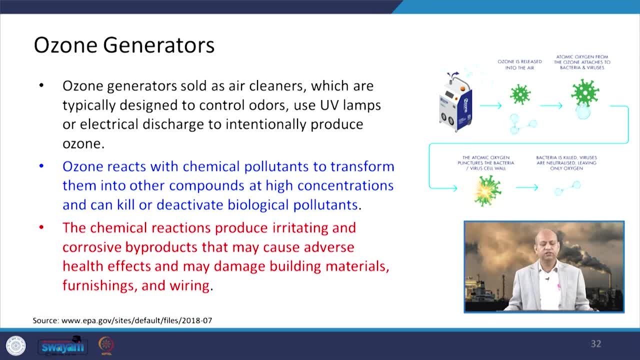 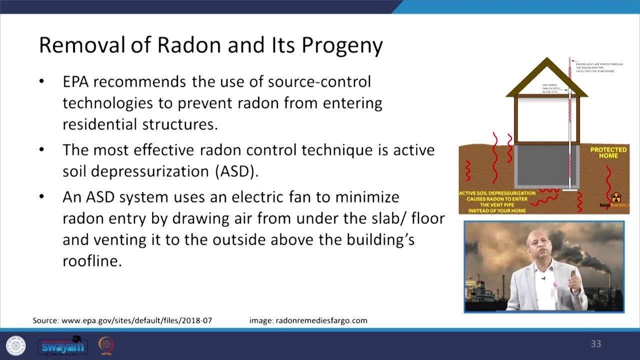 So, again, we have to be careful and we need to handle it with the caution Well then, when we talk about removal of radon and its progeny. so the Environmental Protection Agency of USA recommends the use of source control technologies to prevent radon from. 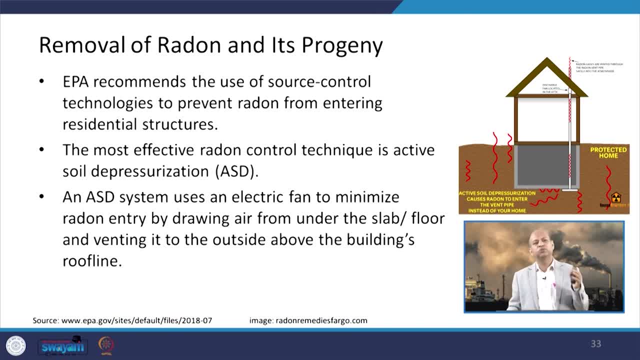 entering residential structures. So the most effective way of controlling the radon technique is active soil. you know this depressurization ASD. So the ASD system uses electric fan to minimize the radon entry by drawing air from under the slab or floor and venting it outside. you know the building, so it does not enter into the. 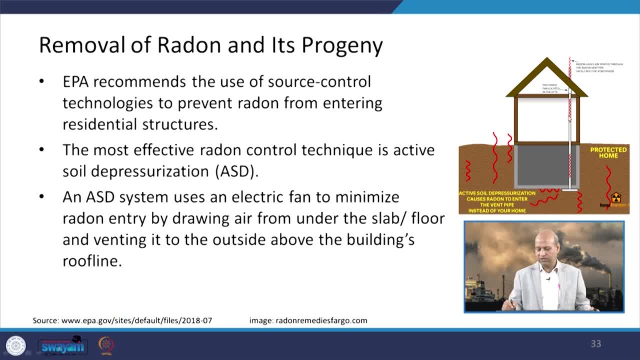 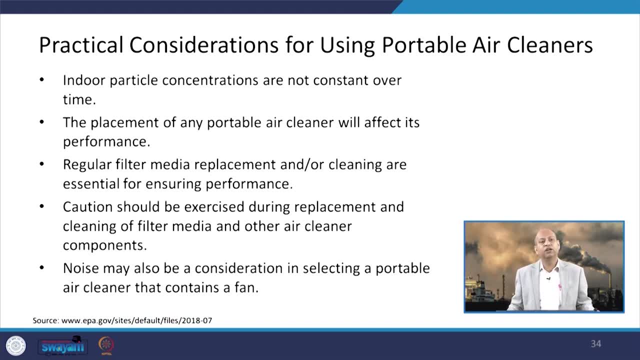 air. You can see here. you know this kind of vents are there and it can take it out, So from subways or those kind of locations. well then, there are practical considerations for portable air cleaners, As I said, because indoor particle concentrations are not constant over time. then the placement: 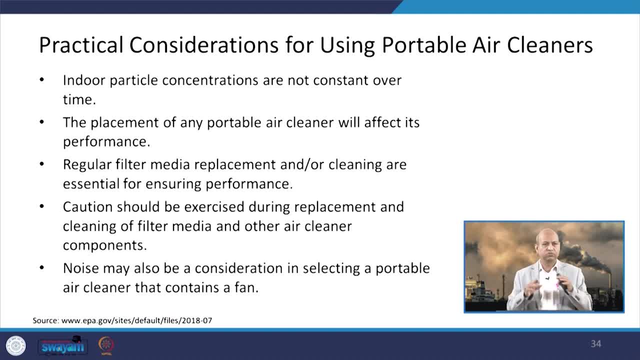 of any portable air cleaner will affect its performance. So we have to be careful where we need to put it so that efficiency is high. Regular filter media replacement is needed, otherwise it will, you know, be source of pollutant rather than cleaning. Replacement or cleaning of the filter media. again, it needs to be handled carefully, otherwise 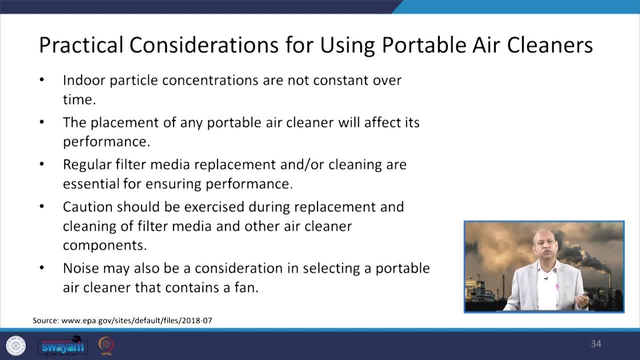 this will add to the pollution. Noise may also be a concern when we are using some particles- Okay, So in particular portable air cleaners. so the noise pollution may be there. so, accordingly, we need to do something so that less noise related portable air cleaners are used. 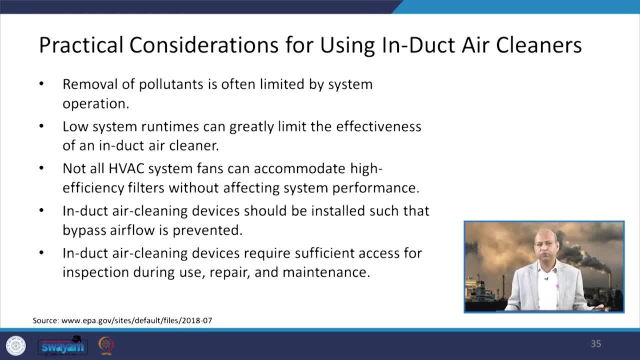 Well then, removal of pollutants is often limited by system operation and the low system. these run times can greatly limit the effectiveness of induct air cleaner. so means the system has to be designed properly so that it has sufficient time. Then not all HVAC systems, you know. 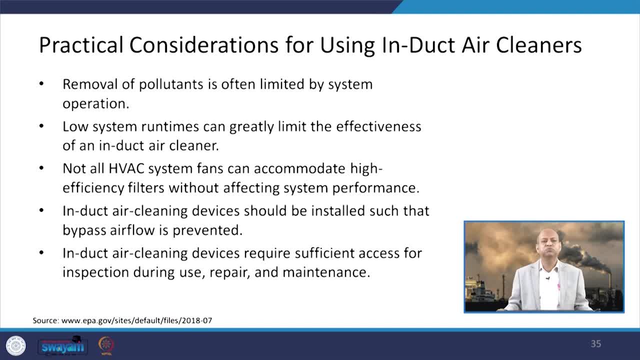 All HVAC systems. you know fans can accommodate high efficiency filters without affecting system performance, So it is a kind of trade-off. you have to see where you can install it and run the HVAC system properly so that it also do air conditioning as well as it removes the pollutants. 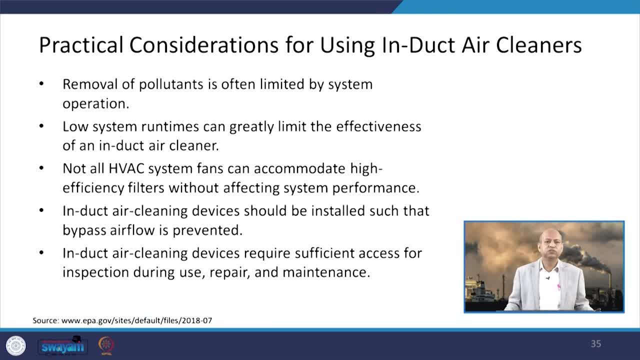 Well induct air cleaning devices. they should be installed such that bypass airflow is prevented. otherwise efficiency will be greatly reduced. and the induct air cleaning devices. they require sufficient access for inspection During use, repair and maintenance. otherwise you know if you do not have a proper access. 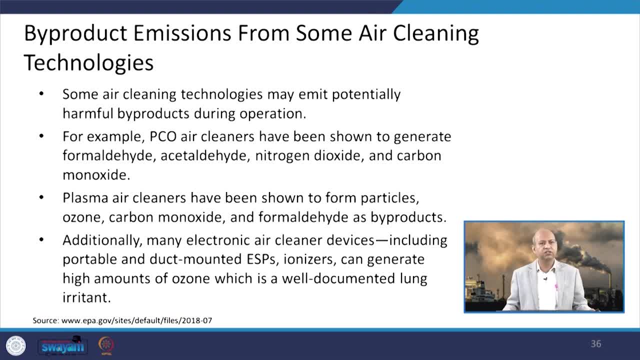 then some kind of pollution accumulation can be there inside the ducts etc. Well, the by-product emissions from some air cleaning technologies can be an issue. So we have to see those technologies as we have seen that in PCO or plasma or ozone related. 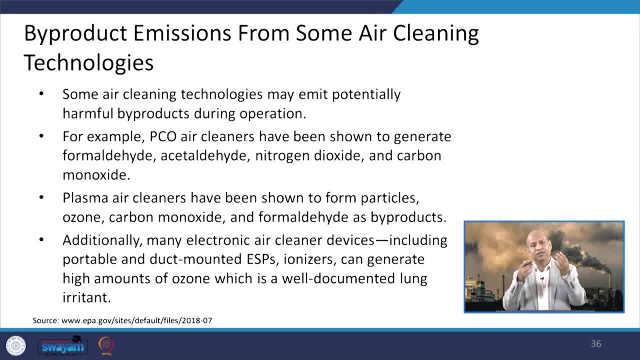 devices. if careful handling is not there, then rather than removing the pollutant, they can add into So some other pollutants like formaldehyde, acetaldehyde. they can be generated in PCO technology. So those things we have to be careful about. 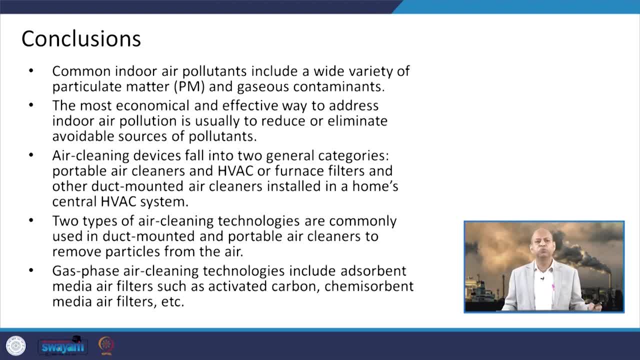 Well, so in conclusion, we can say that the common indoor air pollutants. they can be removed in terms of particulate matter or gaseous contaminants by certain technologies, Depending upon particulate matter is more or gaseous pollutant is more. you can select. 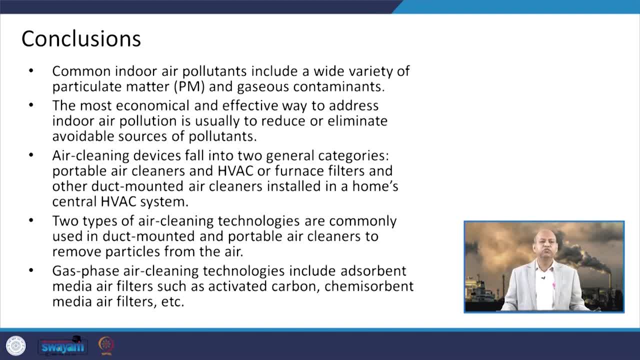 the technology right and the most economical and effective way to address the indoor air pollutant is usually to reduce or eliminate the sources itself, at the source pollutants we have to remove. Then air cleaning devices. you know they can be of two general categories: portable air cleaning and HVAC or furnace filters, which we have seen just now, and they can be mounted.